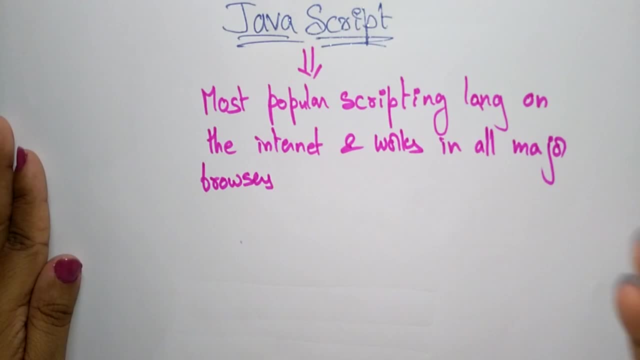 So all major browsers, All the major browser browsers, it will work. It was designed to add interactivity to HTML pages. So whatever the HTML pages you are created, that is a static pages. So to make that HTML pages interactive, you need to use a JavaScript. 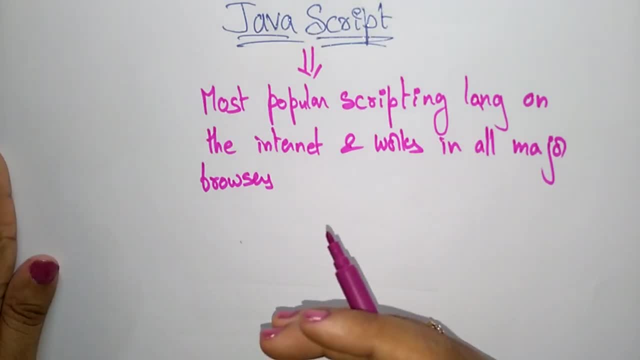 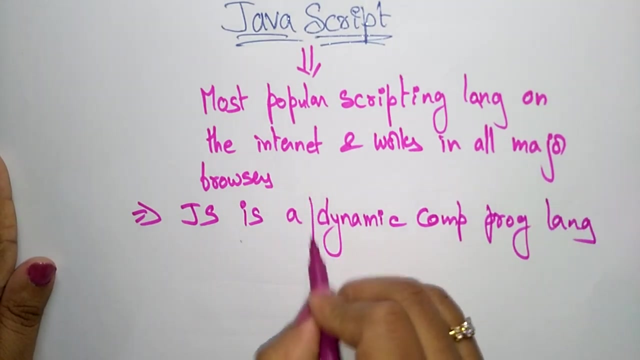 So JavaScript is a dynamic computer programming language. I said HTML is a static language And whereas let me write JavaScript, Yes is a JavaScript. JavaScript is a dynamic computer programming language. So don't forget, this is a dynamic Dynamic means it is giving some interactions. 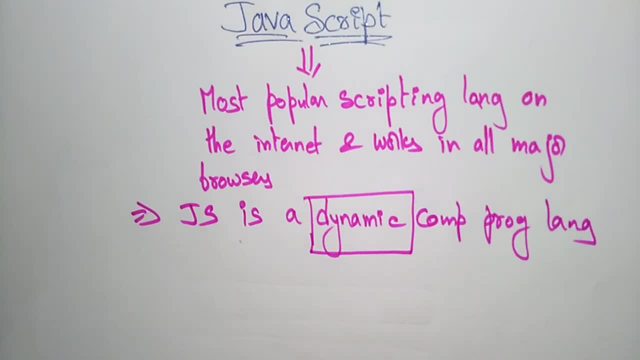 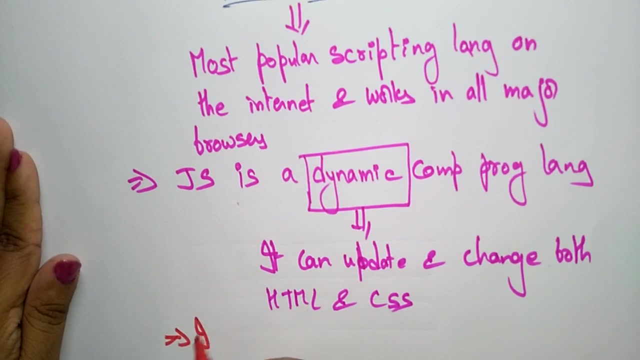 It is providing some interactions on the pages. Okay, So for the web, it can. That means it can update. It can update and change both HTML and cascading style sheets, And it can also use it to calculate, manipulate and validate the data. 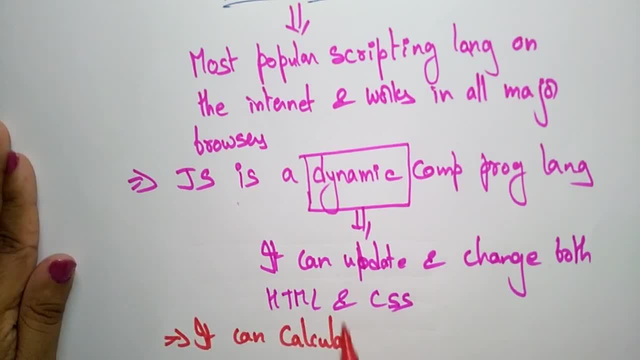 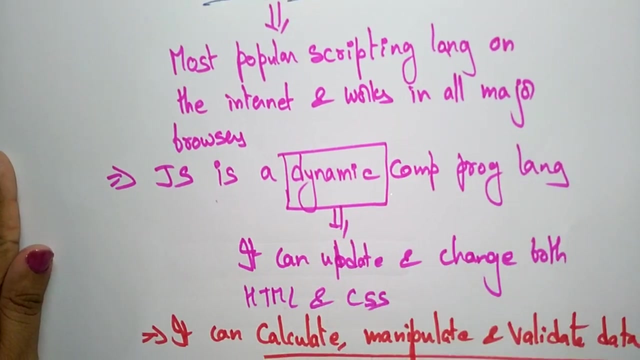 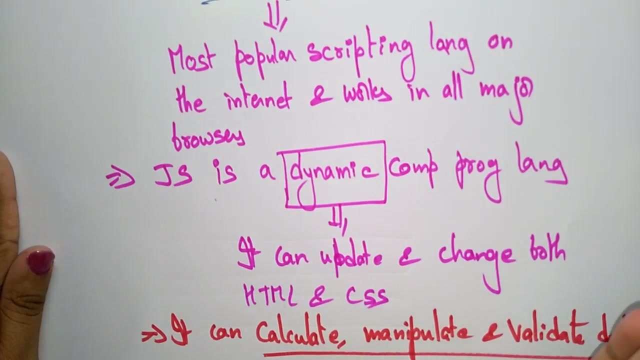 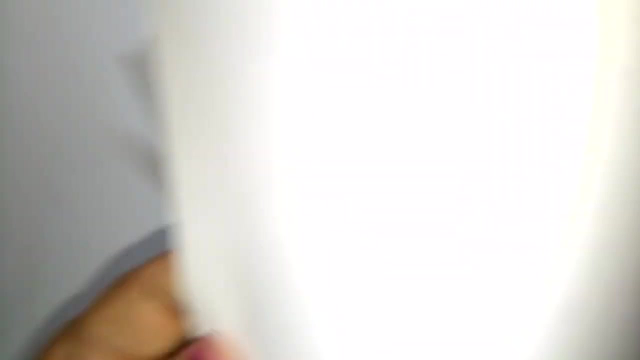 It can calculate, Manipulate And validate data. So that's why we call it as a dynamic computer programming language. A JavaScript is a dynamic computer programming language because it is going to calculate the data, manipulate the data and validate the data. So you can put JavaScript on either of the sections, like: 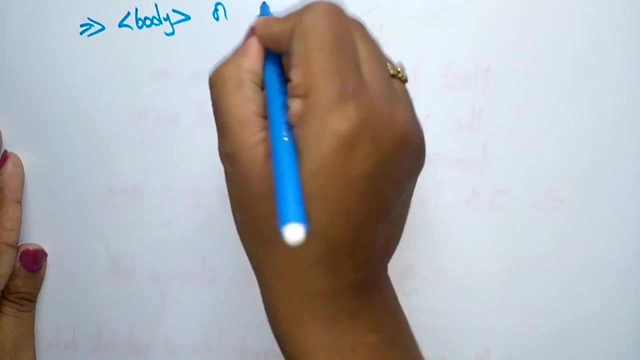 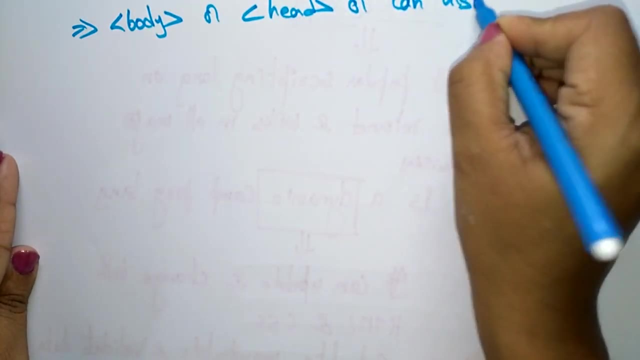 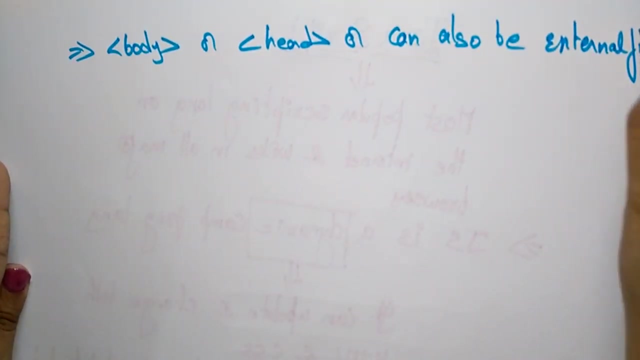 In the body section Or in head section, Or can also be an external file, Or can also be External, External file. So a JavaScript can be right in the body section of HTML or in the head section of HTML, Or you can write some external file. 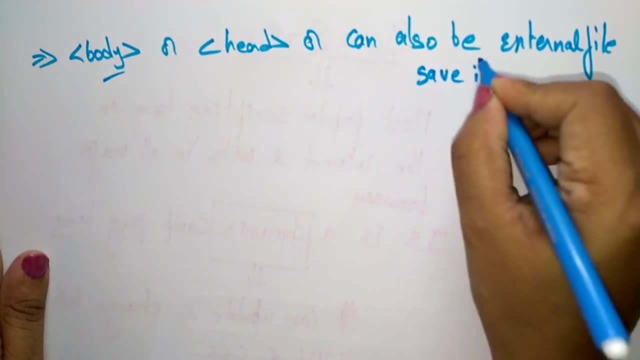 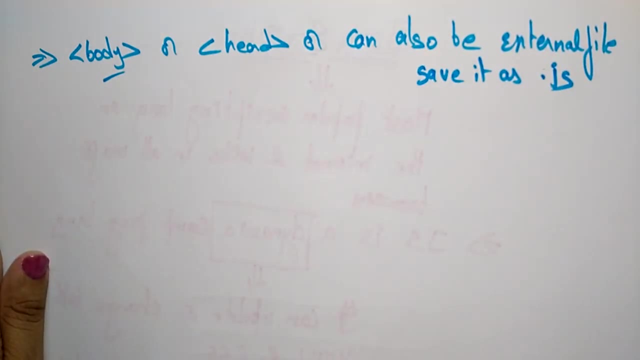 Just save it as a. Save it as js file. So, whereas HTML, you're going to save it as a html. And for JavaScript, if you are using the external file, then save that file as a js file. So let me explain a simple program. 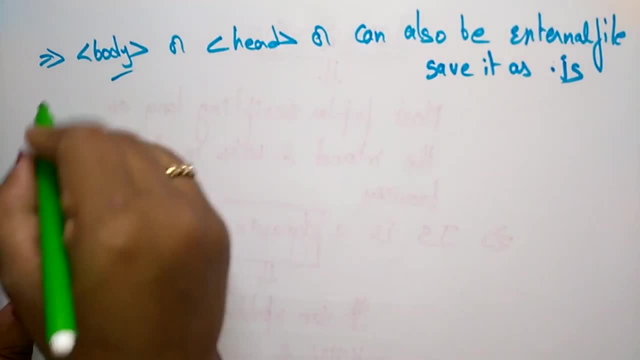 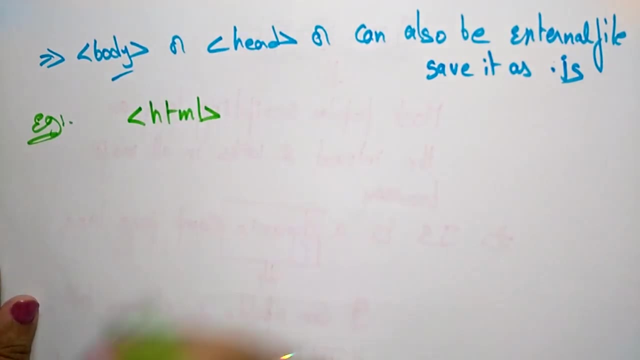 The tags that are present in the JavaScript. I'm just taking a simple program. First let me write the program. After that Let me explain what exactly the each statement was, html. Now here I'm writing the scripting language. That is a JavaScript in body section. 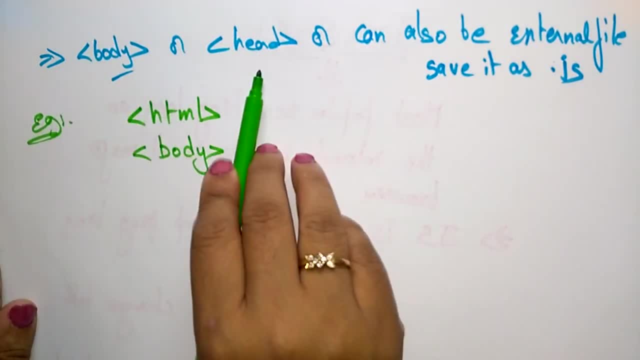 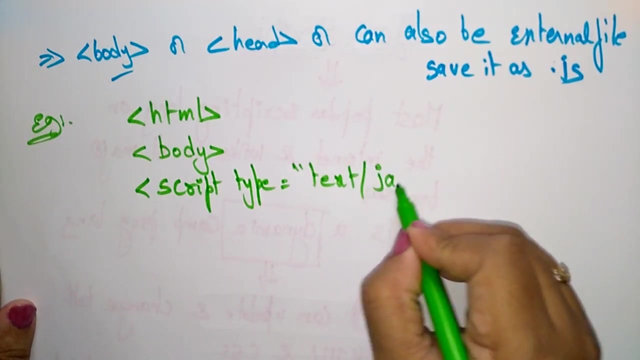 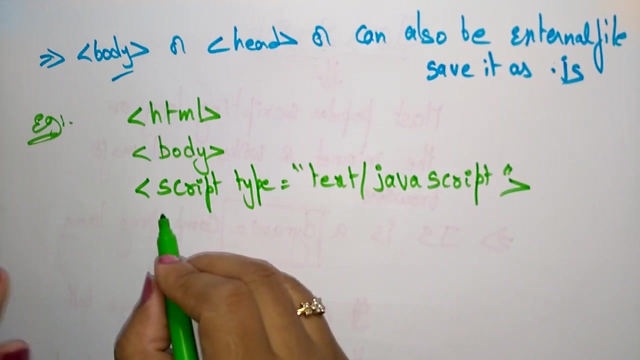 So I said you can write the script language in body or in head or in external file. So now I'm writing in the body. Script Type is equal to It may be a text or a JavaScript Document. I'm not closing the script. 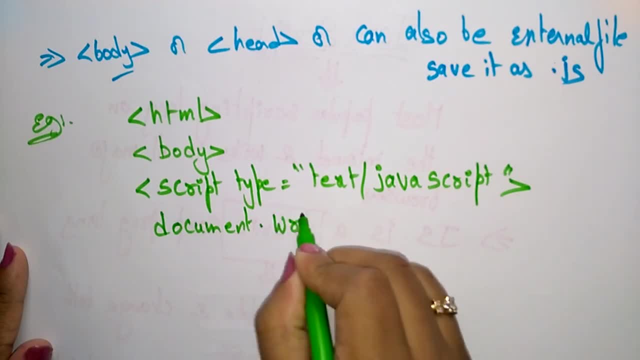 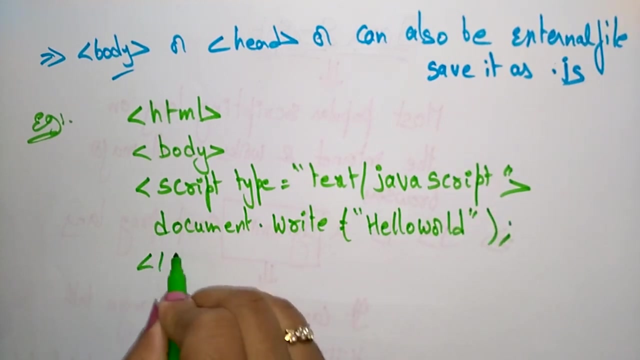 Okay, Document Write is equal to, Or else document Write It may be. Let's take hello world. The message has to be print on the screen: Hello world. Now I'm closing the script tag. After that, I'm closing the body tag. 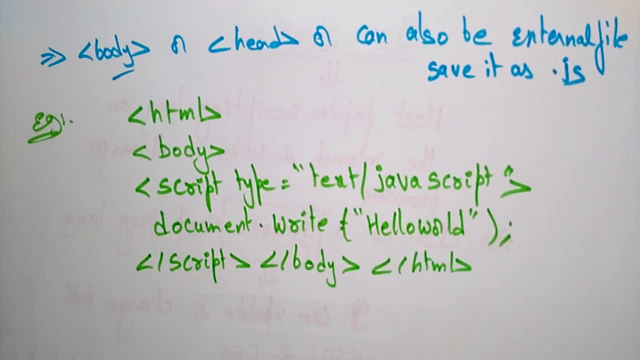 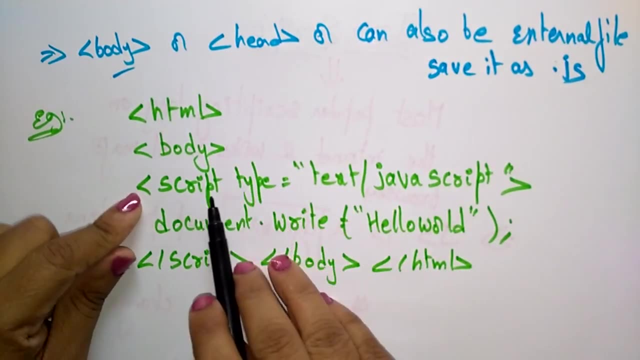 And finally HTML tag. So here I have written a simple program. Let's see what is this. So you know the HTML tags and the body tag. Now let's see what is this. A script type is equal to text or JavaScript. 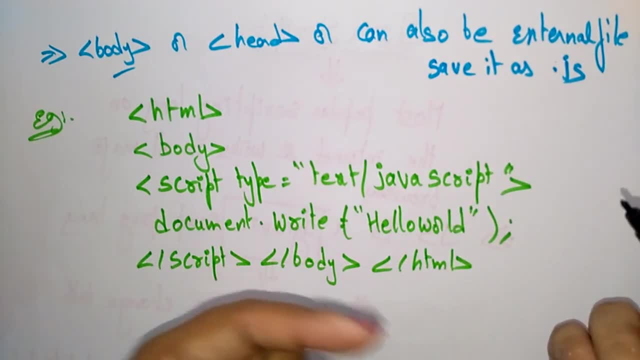 So, whatever the script I'm writing, that script may be a text or a JavaScript. So here the type of a script you will be adding: Either you can add the text or you can add the JavaScript. Now let's see The documentwrite. 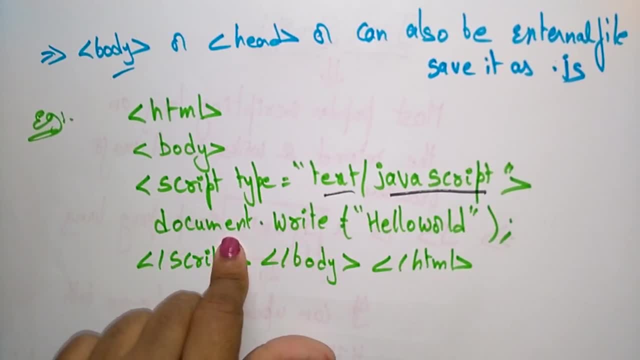 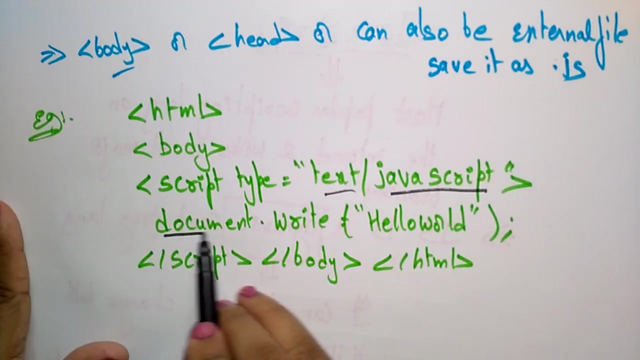 What does the statements indicate? So it tells the page to write the word hello world. So, whatever the web page it is in, So it is telling to the web page to just write the print the word hello world on web page. So this is a standard JavaScript command.